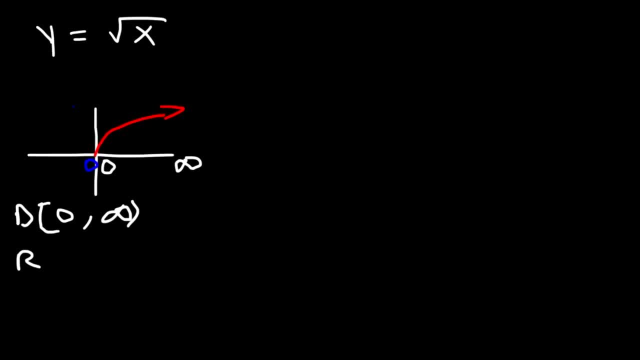 The lowest y value is 0 and the highest is infinity, So the range is also 0 to infinity. So that's the graph of y equals the square root of x. What's the general shape for a negative square root X? What's going to happen if we put a negative sign in front of the radical, If? 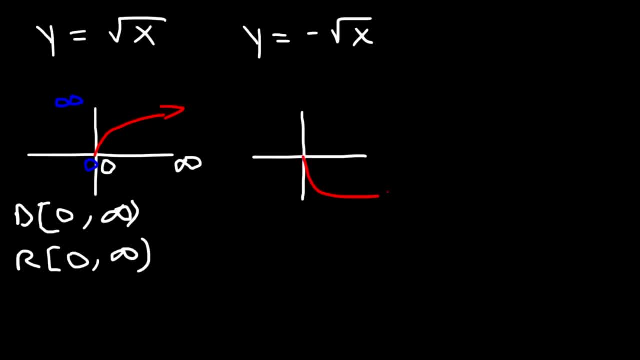 you put a negative sign in front of it, it's going to reflect over the x-axis, So it's going to look like that. And if you put a negative sign inside the radical in front of x, then it's going to reflect over the y-axis. Now if you put, let's say, 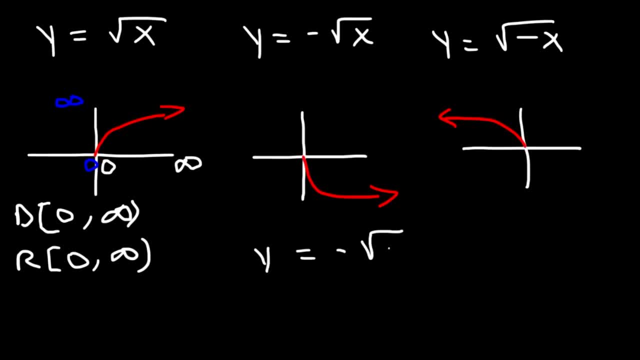 two negative signs, one in front and on the inside of the square root function. this is going to reflect over the origin, And so it's going to look like this. Now, if you have a difficult time remembering all these rules, here's something that can help you: The. 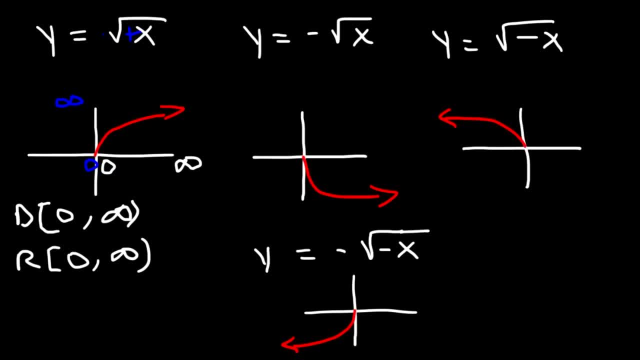 sign in front of x is positive and the sign that's in front of the radical, which we'll say is associated with y, is also positive. X is positive in quadrants 1 and 4.. Y is positive in quadrants 1 and 2.. X and y are both positive in quadrant 1.. So 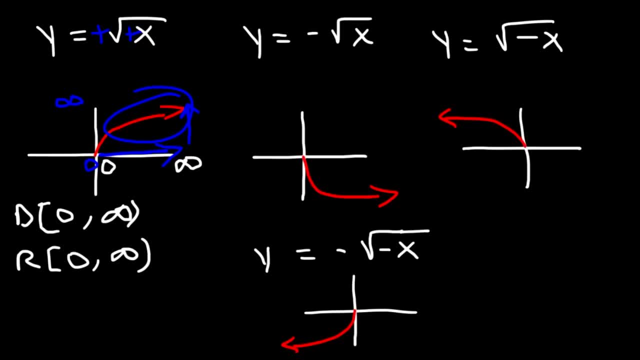 notice that the graph points towards quadrant 1.. So, just so you know, this is quadrant 1.. Here's number 2.. This is quadrant 3 and quadrant 4.. So, looking at the second one, x is positive, y is negative, 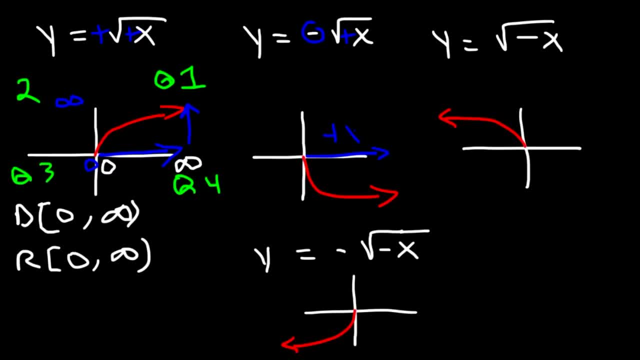 X is positive towards the right, y is negative below the x-axis, So it points towards quadrant 4.. Now, looking at the third example, x is negative, y is positive, X is negative towards the left, y is positive above the x-axis, So it's: 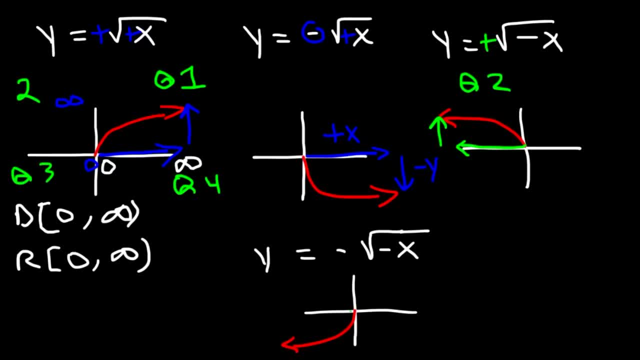 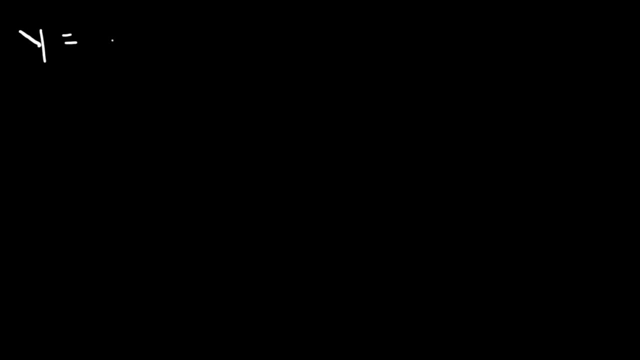 going to go towards quadrant 2.. And for the last example, x is negative towards the left, y is negative below, and so it goes towards quadrant 4.. That can help you to determine what direction the graph is going to go. Now, what about this example? What's going to happen if we add 2 to the square root of? 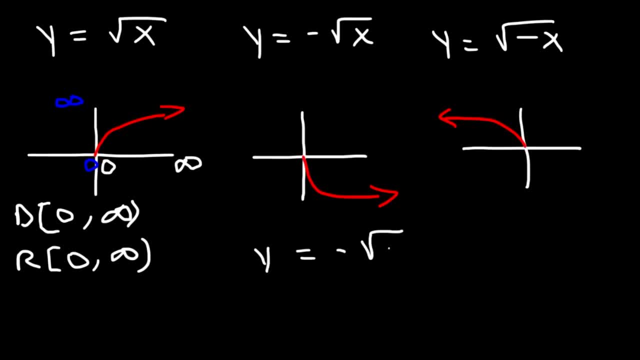 two negative signs, one in front and on the inside of the square root function. this is going to reflect over the origin, And so it's going to look like this. Now, if you have a difficult time remembering all these rules, here's something that can help you: The. 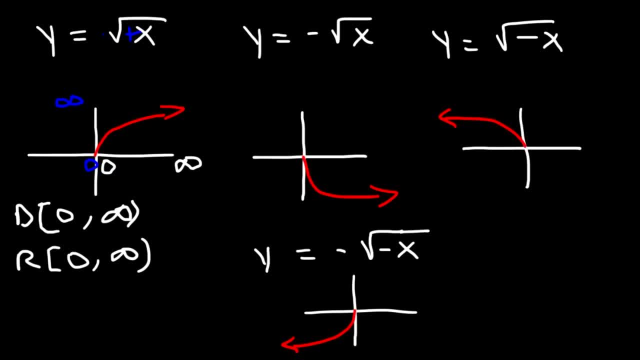 sign in front of x is positive and the sign that's in front of the radical, which we'll say is associated with y, is also positive. X is positive in quadrants 1 and 4.. Y is positive in quadrants 1 and 2.. X and y are both positive in quadrant 1.. So 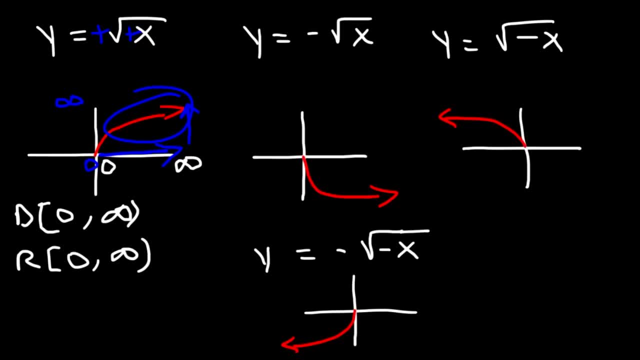 notice that the graph points towards quadrant 1.. So, just so you know, this is quadrant 1.. Here's number 2.. This is quadrant 3 and quadrant 4.. So, looking at the second one, x is positive, y is negative, 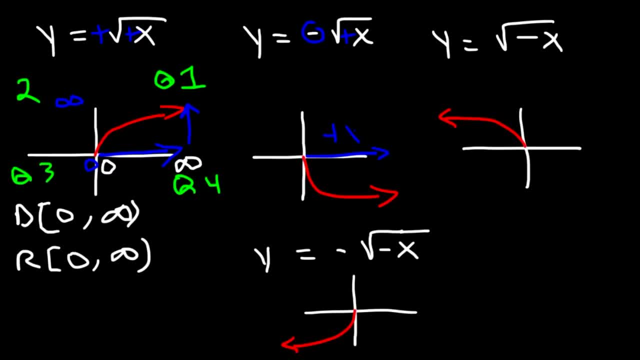 X is positive towards the right, y is negative below the x-axis, So it points towards quadrant 4.. Now, looking at the third example, x is negative, y is positive, X is negative towards the left, y is positive above the x-axis, So it's: 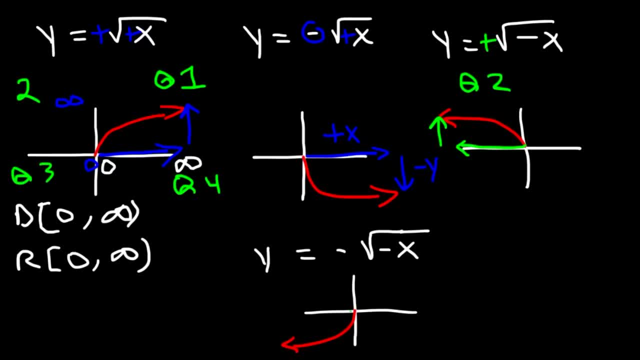 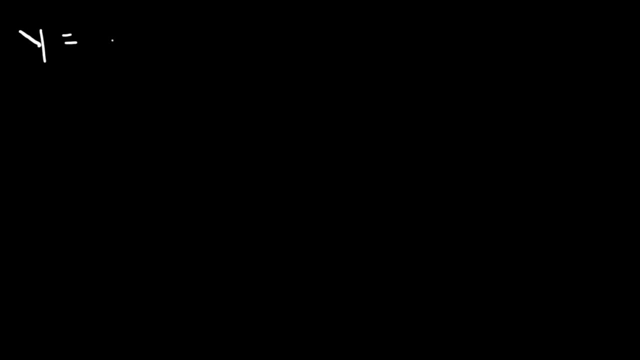 going to go towards quadrant 2.. And for the last example, x is negative towards the left, y is negative below, and so it goes towards quadrant 4.. That can help you to determine what direction the graph is going to go. Now, what about this example? What's going to happen if we add 2 to the square root of? 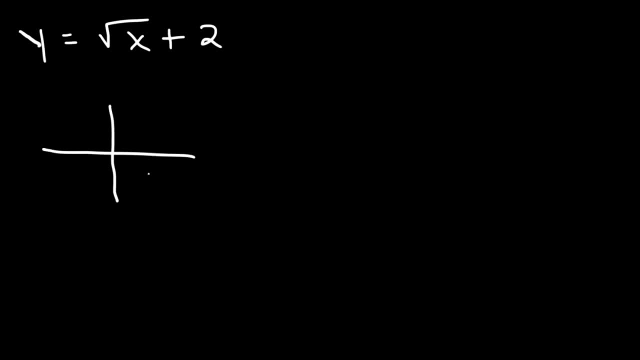 x. How is it going to affect the graph? In this case, the graph is going to start 2 units above the x-axis, So it's shifted up 2 units. Now if we were to, let's say, subtract it by 1, it's going to shift down 1 unit, But it's still going to go towards. 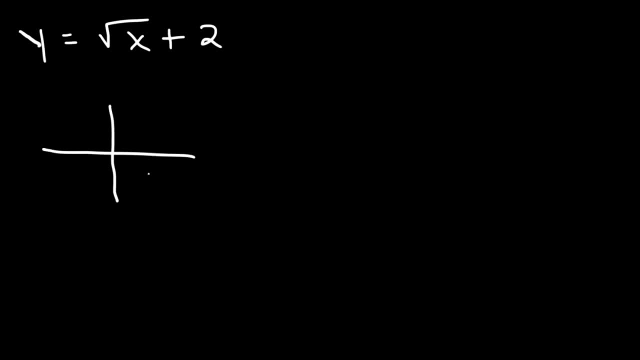 x. How is it going to affect the graph? In this case, the graph is going to start 2 units above the x-axis, So it's shifted up 2 units. Now if we were to, let's say, subtract it by 1, it's going to shift down 1 unit, But it's still going to go towards. 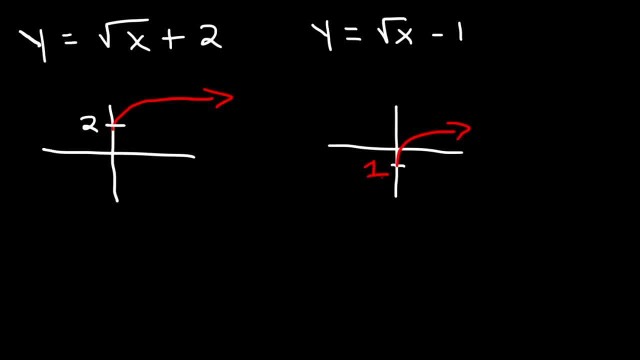 quadrant 1.. So it looks like that. Now, what about this graph? Let's say, if we have the square root of x minus 2.. In this case it's going to shift to the right 2 units. What you can do is set the inside equal to 0 and solve for x. 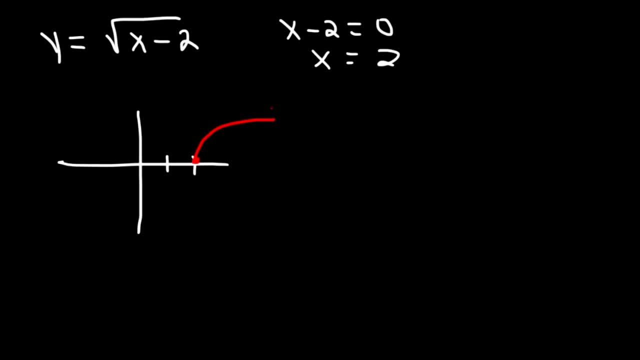 In that case, it's going to start 2 units to the right and it's going to go this way. So likewise, let's say, if we have the square root of x plus 3, the graph is going to be shifted 3 units to the left and it's going to open towards the right. 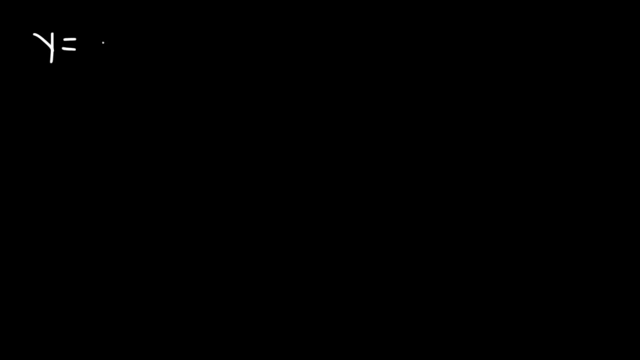 Now let's draw a more accurate sketch using points. Let's graph these two functions. So for the first one, the first point starts at the origin. It's Now to find the next point. it's important to understand that the square root of 1 is 1.. So, starting, 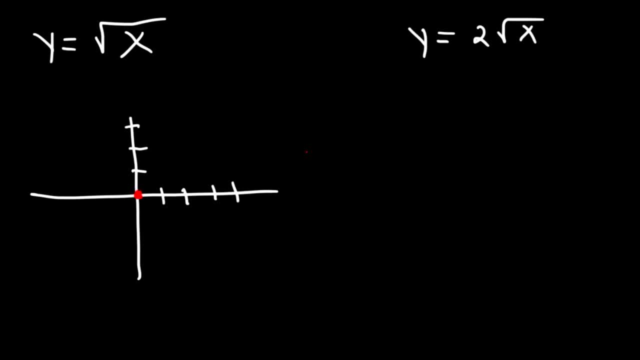 from the origin, as you travel 1 to the right, go up 1 unit. Now the square root of 4 is 2.. Starting from the origin, as you travel 4 to the right, you need to travel up 2 units. 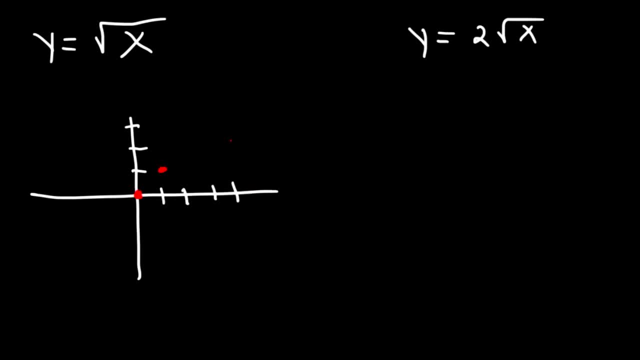 So therefore, the next point is going to be: The square root of 9 is 3, so if you want another point, you can plot. I think this is good enough And that's how you can get a more accurate sketch. 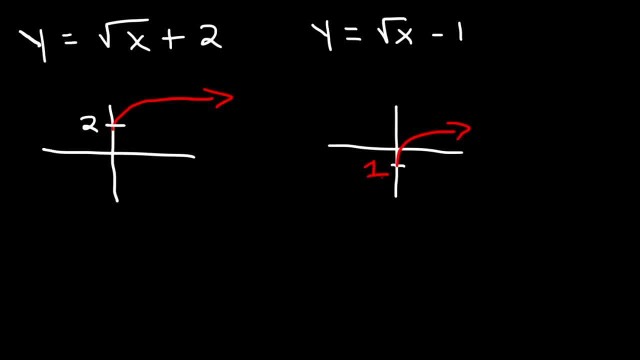 quadrant 1.. So it looks like that. Now, what about this graph? Let's say, if we have the square root of x minus 2.. In this case it's going to shift to the right 2 units. What you can do is set the inside equal to 0 and solve for x. 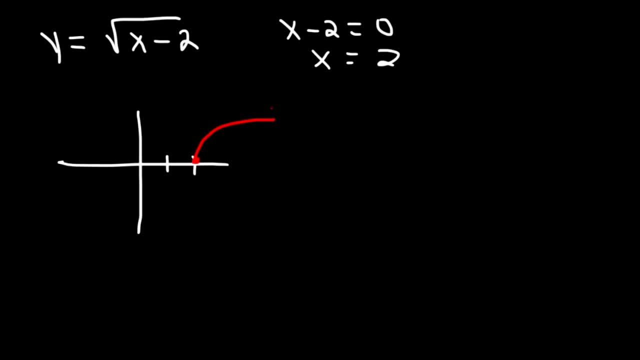 In that case, it's going to start 2 units to the right and it's going to go this way. So likewise, let's say, if we have the square root of x plus 3, the graph is going to be shifted 3 units to the left and it's going to open towards the right. 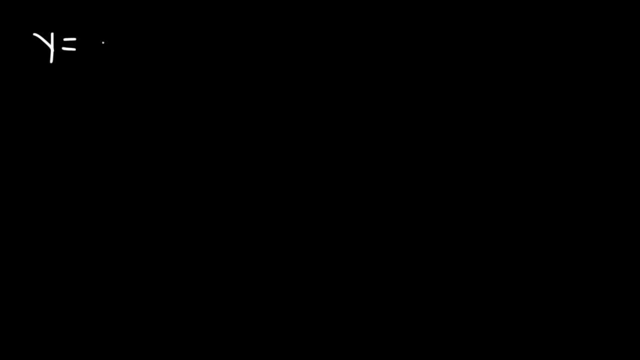 Now let's draw a more accurate sketch using points. Let's graph these two functions. So for the first one, the first point starts at the origin. it's a 0, 0.. Now to find the next point. it's important to understand that the square 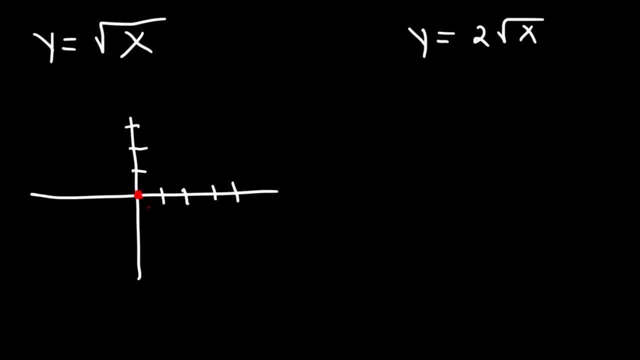 root of 1 is 1.. So, starting from the origin, as you travel, one to the right, go up one unit. Now the square root of four is two. So, Starting from the origin, as you travel 4 to the right, you need to travel up 2 units. 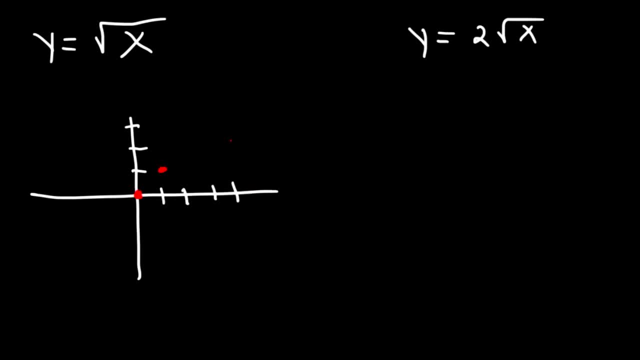 So therefore, the next point is going to be: The square root of 9 is 3, so if you want another point, you can plot. I think this is good enough And that's how you can get a more accurate sketch. 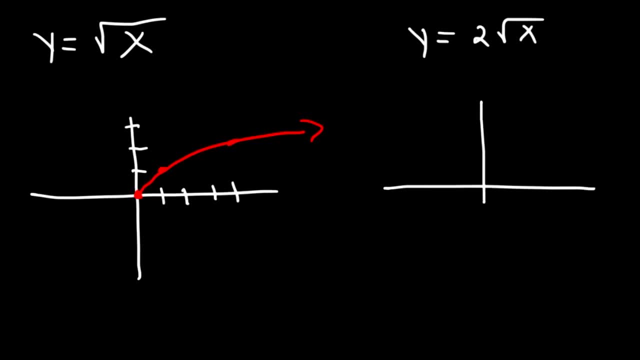 So let's see what happens if we put a 2 in front of the square root. Now everything is going to be the same. the only difference is the y values will double. So the origin is going to be the same. Now, as we travel 1 to the right, instead of going up 1, we need to double the up 1 part. 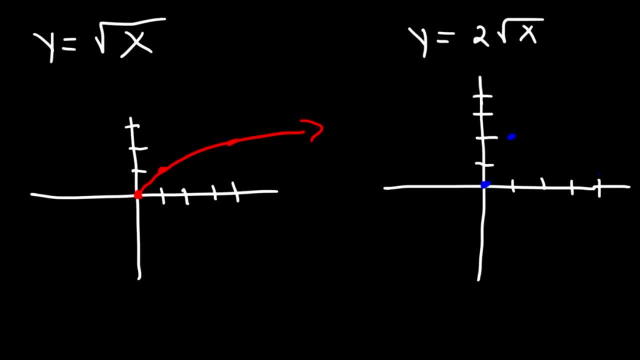 it's going to go up 2.. As we travel 4 units to the right, instead of going up 2, we're going to go up 2.. We're going to go up 4, relative to the origin. So this graph is going to look like this. 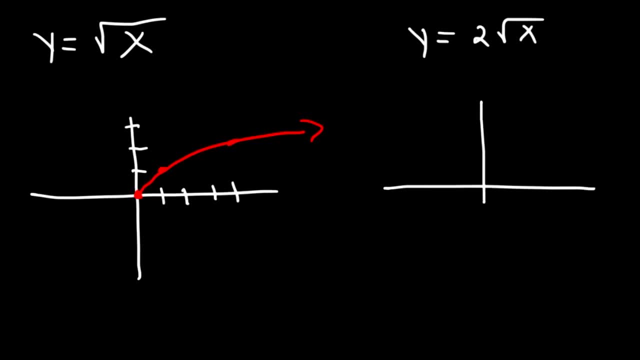 So let's see what happens if we put a 2 in front of the square root. Now everything is going to be the same. the only difference is the y values will double. So the origin is going to be the same. Now, as we travel 1 to the right, instead of going up 1, we need to double the up 1 part. 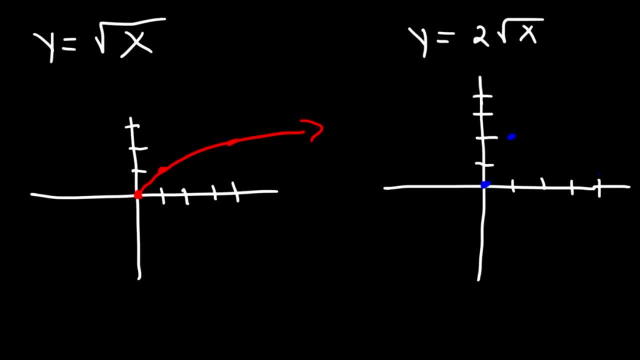 it's going to go up 2.. As we travel 4 units to the right, instead of going up 2, we're going to go up 2.. We're going to go up 4, relative to the origin. So this graph is going to look like this. 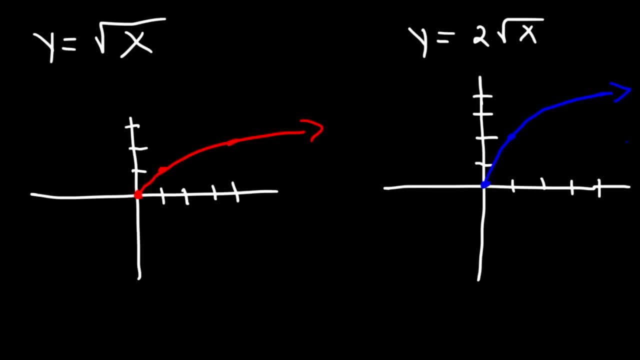 As you can see, it's been stretched vertically by a factor of 2.. Now let's say, if we have this function, the square root of plus 2.. So you can plot points if you want to, but what I want you to do is graph it and also. 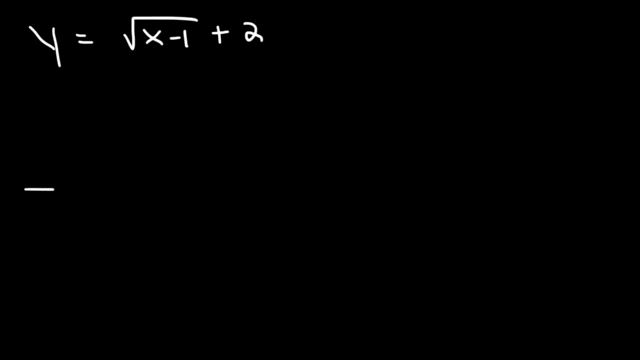 write the domain and range of the function. So first let's find the new origin. The graph has been shifted 1 unit to the right and it's been shifted up 2 units. So therefore we're going to start at. 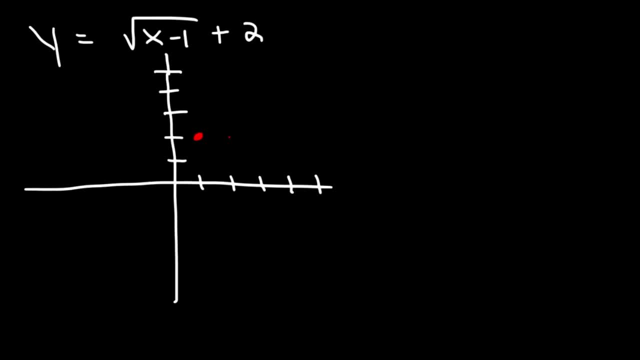 Now to find the next point. as we travel 1 to the right, we need to go up 1 unit, So that's going to take us to. And if we travel 4 to the right, it's going to go up 2 units, so that's going to take. 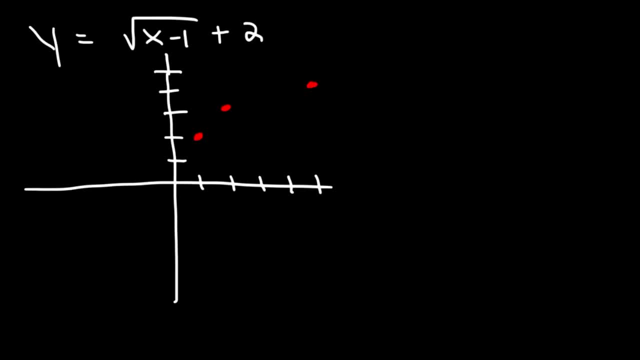 us to, And so those are the points that we have, And the graph is going to go like that. So now to analyze the domain of the function, we need to look at the x values. The lowest x value is 1,. the highest is infinity. 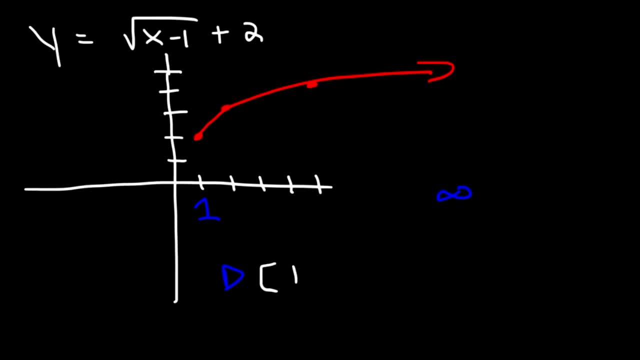 Therefore, the domain is going to be 1 to infinity and it includes 1.. So we need to use a bracket with 1.. For infinity, always use parentheses. Now let's analyze the range. The lowest y value is 2, and the highest goes up to infinity. 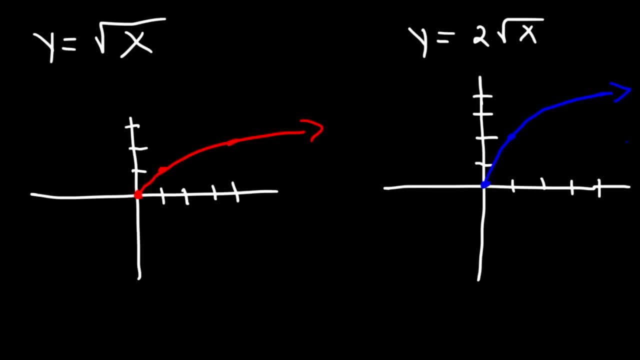 As you can see, it's been stretched vertically by a factor of 2.. Now let's say, if we have this function, the square root of plus 2.. So you can plot points if you want to, but what I want you to do is graph it and also. 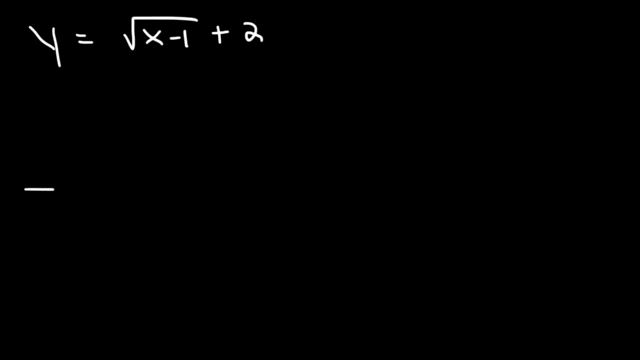 write the domain and range of the function. So first let's find the new origin. The graph has been shifted 1 unit to the right and it's been shifted up 2 units. So therefore we're going to start at. 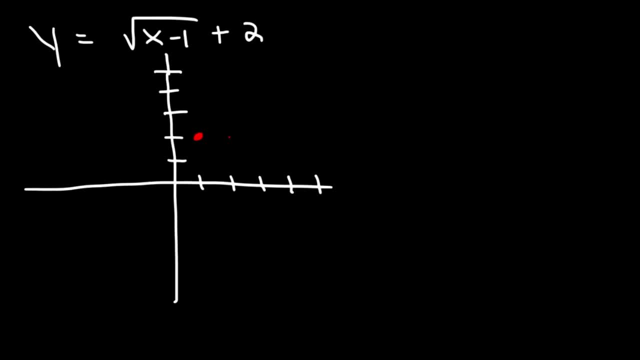 Now to find the next point. as we travel 1 to the right, we need to go up 1 unit, So that's going to take us to comma 3.. And if we travel 4 to the right, it's going to go up 2 units, so that's going to take. 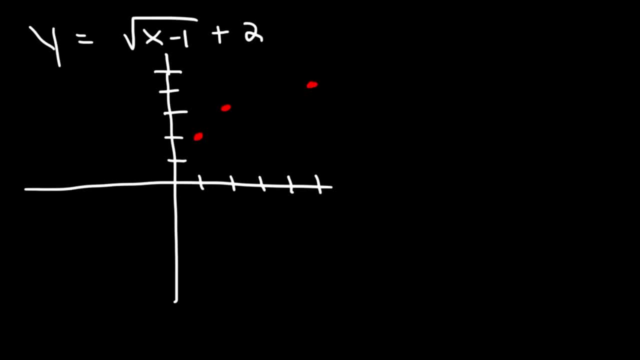 us to 5 comma 4.. And so those are the points that we have, And the graph is going to go like that. So now, to analyze the domain of the function, we need to look at the x values, The lowest x value. 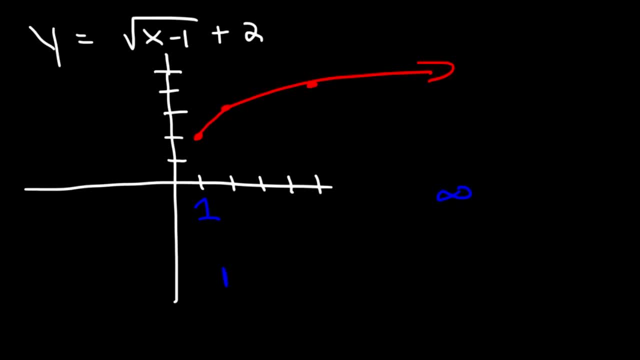 is 1.. The highest is infinity. Therefore, the domain is going to be 1 to infinity, And it includes 1, so we need to use a bracket with 1.. For infinity, always use parentheses. Now let's analyze the range. The lowest y value is 2, and the highest goes up to infinity. So therefore, 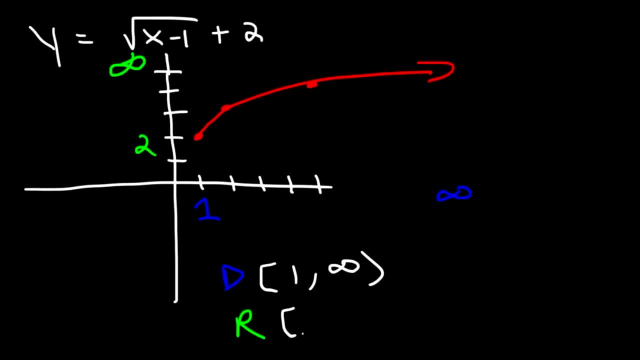 the range is going to be 2 to infinity. So now let's work on another example. Try this one. Let's say that y is equal to 3.. 3 minus the square root of x minus 4.. Go ahead and graph it and then write the domain and. 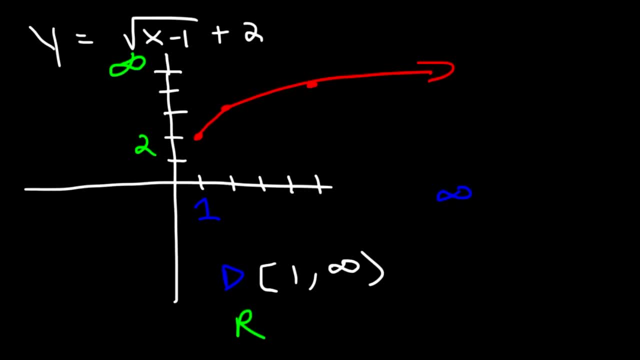 So therefore, the range is going to be 2 to infinity. So now let's work on another example. Try this one. Let's say that y is equal to 3 minus the square root of infinity. So now let's analyze the range. 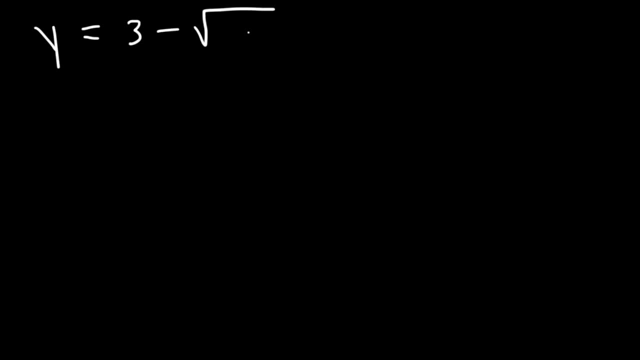 The lowest y value is 2, and the highest goes up to infinity. Therefore, the range is going to be 2 to infinity. His is the square root of x minus 4.. Go ahead and graph it and then write the domain and range of the function using interval notation. 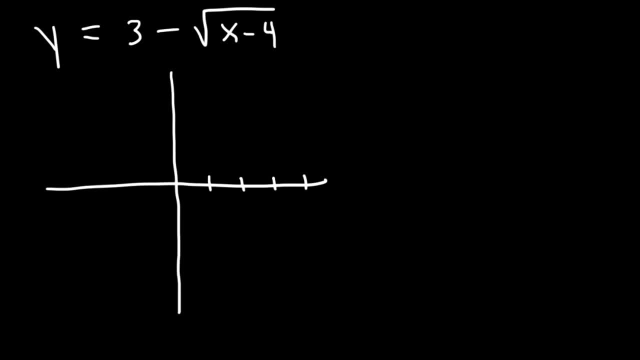 So we can see that the graph has shifted 4 units to the right And its been shifted up three. If you want to, you can rewrite it like this: 1 to infinity And y to infinity, 4 to infinity, 1 to infinity. 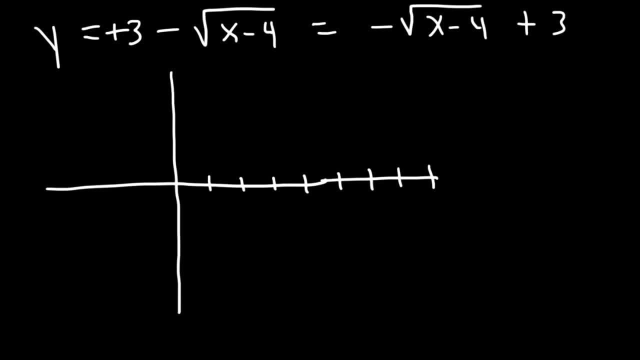 1 to infinity, If that makes it easier. Now there is a negative sign in front of the radical, So it's not going to be going towards quadrant 1.. Rather, it's going towards quadrant 2.. X is positive. 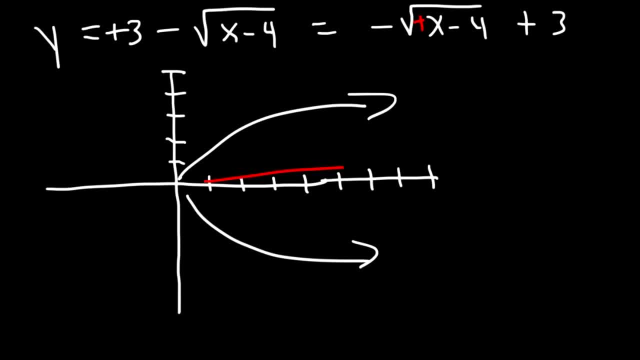 Since there's a positive sign in front of X, so it's going to go towards the right, But since there's a negative on the outside, Y is negative, So it's going to go towards quadrant 4.. But now let's find a new origin. 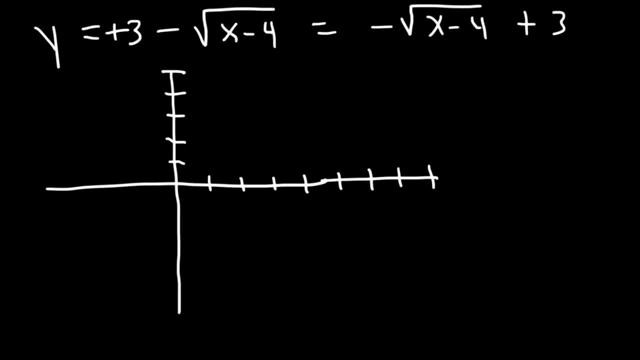 So the graph has been shifted 4 to the right and 3 units up. So it starts at this point 4,3.. And we know that the graph is going to go towards quadrant 4.. So when we find the next point, as we travel, 1 unit to the right. 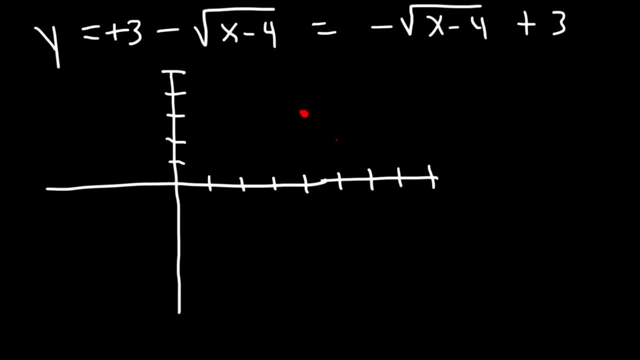 instead of it going up 1 unit, we need to go down 1 unit due to the negative sign. So that's going to take us to the point 5,2.. And since the square root of 4 is 2,, as we travel 4 to the right, we need to go down 2.. 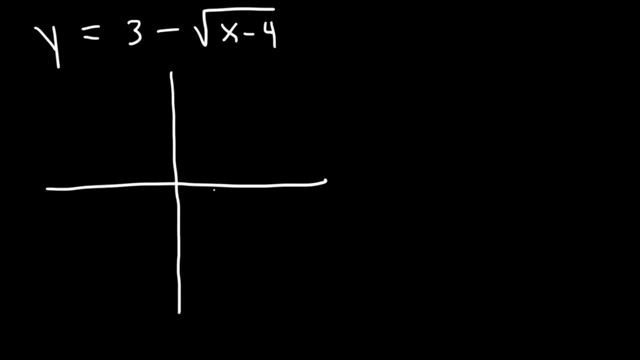 range of the function using interval notation. So we can see that the graph has shifted 4 units to the right And it's been shifted up 3.. If you want to, you can rewrite it like this, If that makes it easier. Now there is a negative sign in front of the radical, So it's not going to. 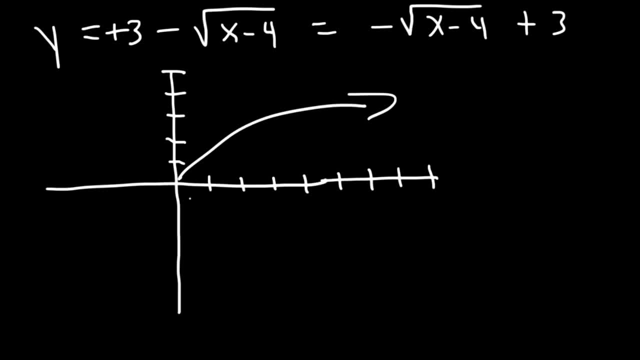 be going towards quadrant 1, rather it's going towards quadrant 2.. X is positive, since there's a positive sign in front of X, so it's going to go towards the right, But since this is a negative on the outside, 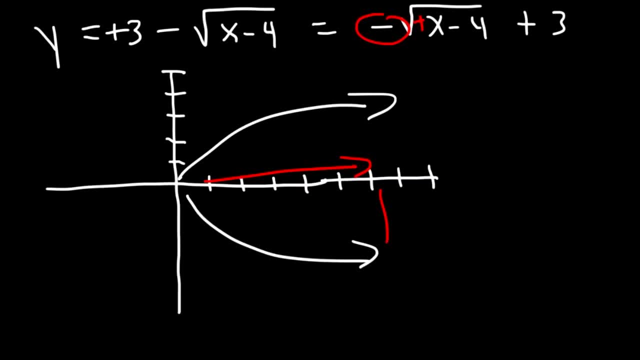 why it's negative. so it's going to go towards quadrant four. but now let's find a new origin. so the graph has been shifted four to the right and three units up. so it starts at this point, four comma three, and we know that the graph is going to go towards quadrant four. so when we find the next point, as we travel, 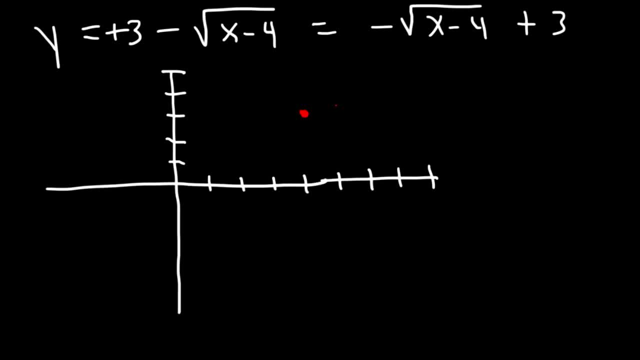 one unit to the right. instead of it going up one unit, we need to go down one unit due to the negative sign. so that's going to take us to the point five, comma two, and since the square root of four is two, as we travel, four to the right, we need. 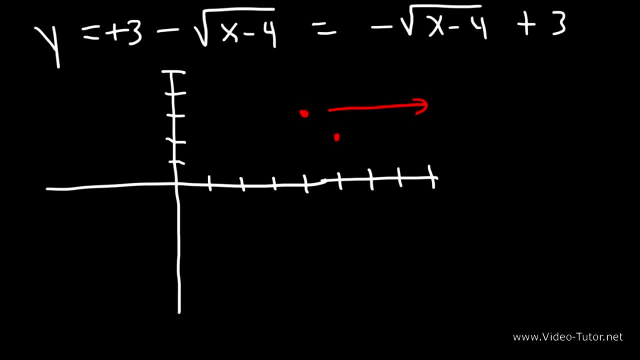 to go down two. so that's going to take us to the point eight, comma one, which is about here, and so this is going to be: let's do that again. here we go. so that's going to be the shape of the graph. so now the domain is going to be four to infinity, since four is the lowest x value. 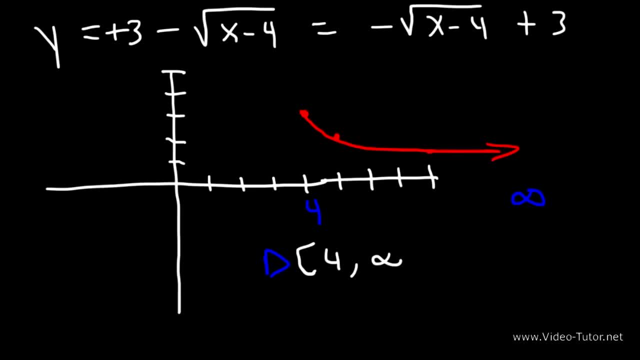 and includes four. and as for the range, the lowest- actually the highest- y value is three. the lowest is negative infinity. as this travels towards the right, it's slowly decreasing, but it continues to decrease forever. so therefore the lowest y value is negative infinity. so the range is going to be from negative infinity to three. including three, and so that's it for this problem.